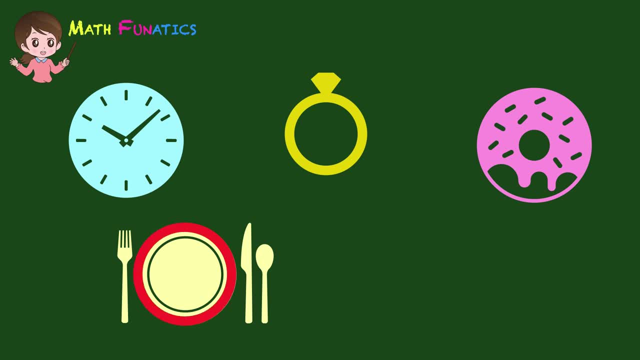 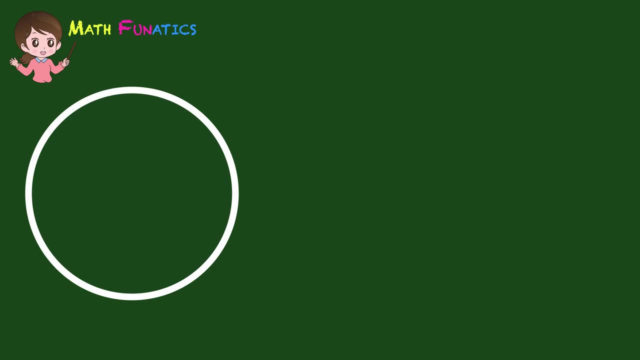 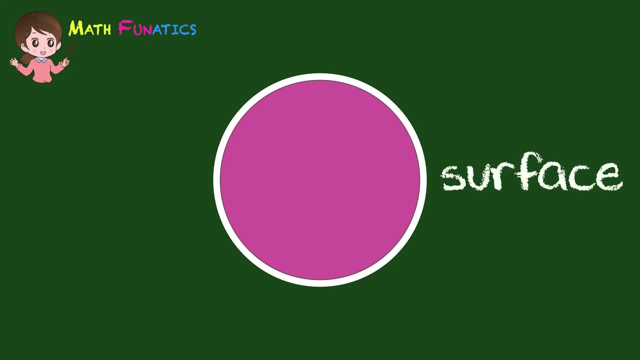 Let us have some examples. This is the shape of a circle, And this motorcycle has two circular wheels. Now let us identify the different parts of a circle. First is the surface. This is the part that is enclosed within the outline of the circle. 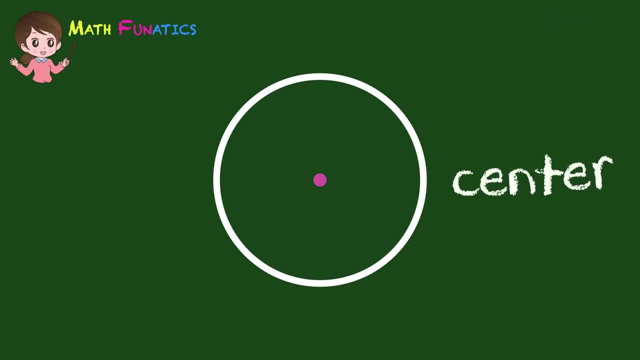 Then we have the center. This is the point that is equidistant from all the points on the circle. This distance from the center to any point on the circle is called the radius. A straight line whose end points both lie on a circle is called the chord. 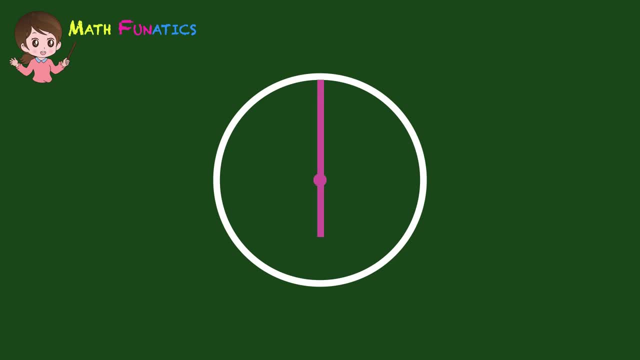 The longest chord in a circle is called the diameter. A diameter is twice a radius. A portion of the outline of a circle is called an arc. A region bounded by a chord of a circle and an inch of a circle is called an arc. 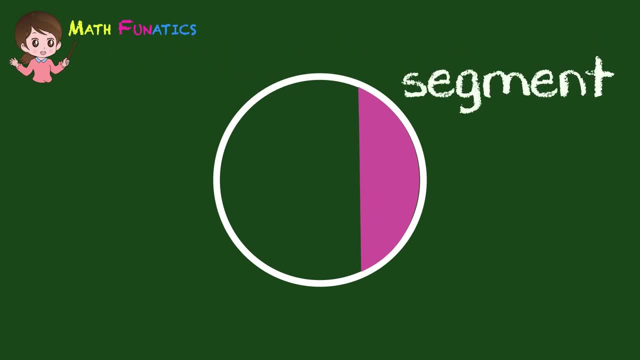 And an intercepted arc is called a segment. A portion that is made of an arc along with its two radii is called a sector. The distance around a circle is called the circumference. Half of the distance around a circle is called semicircle.